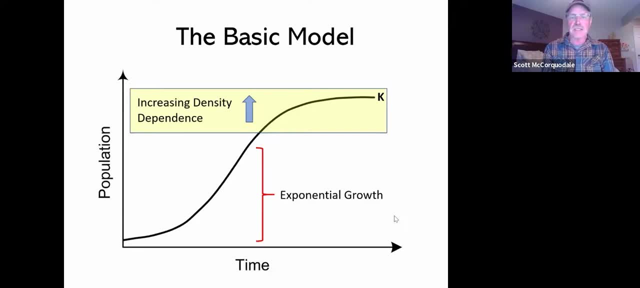 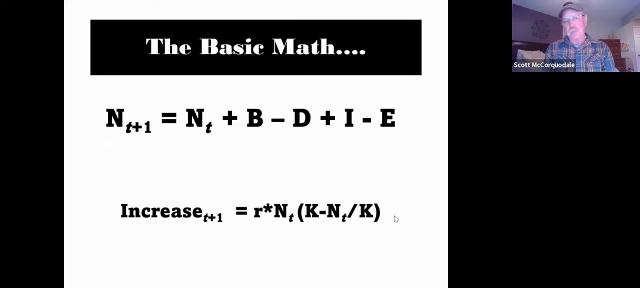 a phenomenon occurring in this yellow box that we call density dependence. So there are things that are happening In the environment and with the animals that changes the way the population is trending through time. So just because this has says math on it, This is really pretty straightforward stuff. So the basic math. 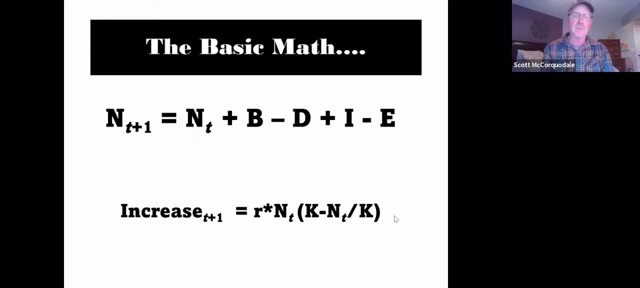 For this is that the number of animals at any future time step is equal to the number of animals at the previous time step, Plus the births, minus the deaths, plus the immigrants Animals that walked in, minus the immigrants animals that walked out, The number of animals that are added each time step. this increase is captured by the second, pretty simple equation on the: 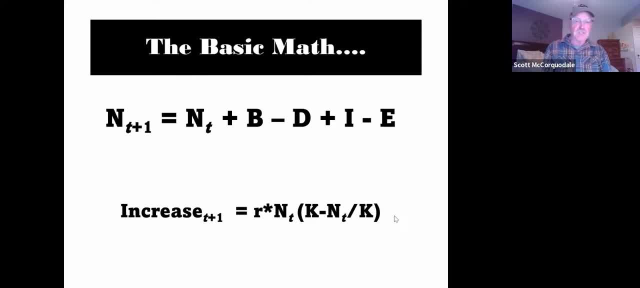 Bottom, where it's the rate times the number of animals at time. T is the increase that will occur over the next time step. but So that's the growth paid. But there's this density dependence penalty. this sort of makes it fit this model, And so the Dennis pens penalty is here, as you can see, is is it's the number of animals on the landscape is really a lot smaller than the carrying capacity, which is k, then this number is going to be really 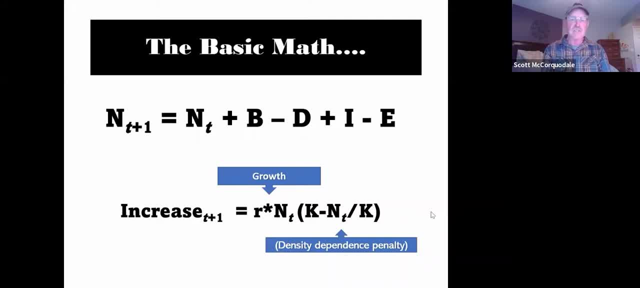 close To one, And so it's really going to be. the growth is just going to be. this are times NT, but if the, if the population is and is really large relative to the eigentlich generally round balance and shoulders- Ok Yeah, relative to k or even more than k- that number is going to turn into a number that's very close, or? 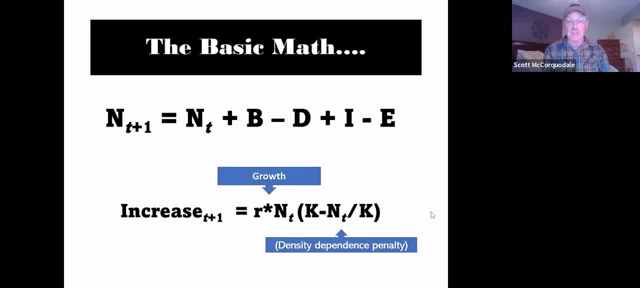 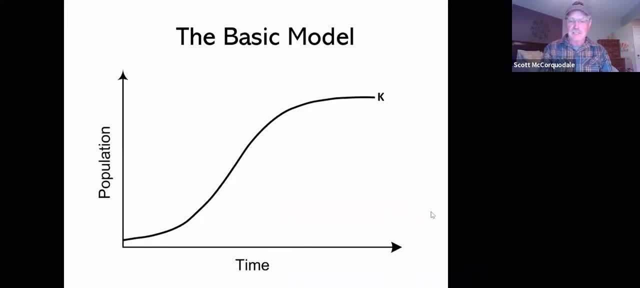 is zero, And so then that basically wipes out the increase completely, because r times nt times zero is zero. So we might describe phases that are associated with this logistic model, So this early phase where there are a small number of animals that are growing but they're not growing. 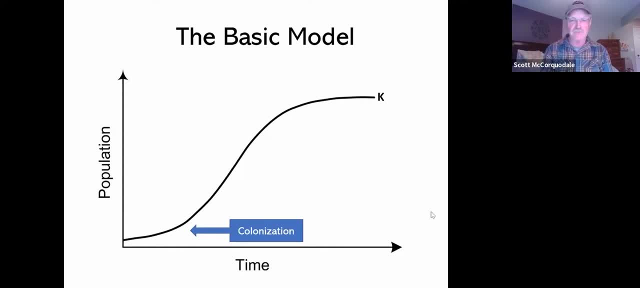 super fast. we would call colonization phase. Then there's this eruption phase where the sort of this exponential function starts to really kick in and you get this really rapid increase in animals or, if it was your bank account, in money And then eventually reach this asymptote which 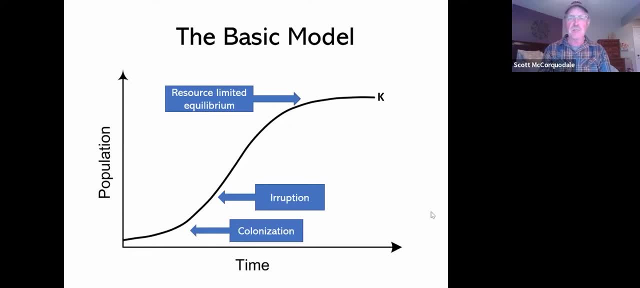 is. we could define that as a resource limited equilibrium, And we'll we're going to sort of flesh all that out in more detail Here in a minute, Just for for just because maybe interesting to people. So you've probably heard the term maximum sustained yield, So maximum sustained yield has really been traditionally. 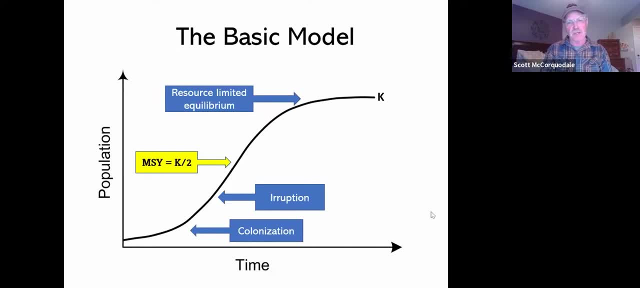 estimated to be about half of the carrying capacity. So be right about there on that curve. So we can kind of think about what is happening with the population as it moves along this curve By pondering what we would expect to see in a variety of sort of parameters, So one would be per capita. 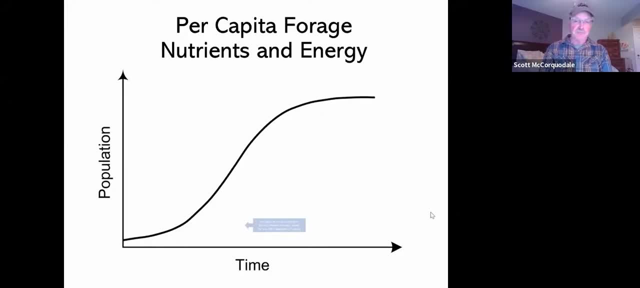 forage, nutrients and energy. So in the colonization phase that is very, very high. There's almost no nutritional limitation. Animals are getting optimal season intake or very close to it, And the specific: the competition between the same species. So animals within this population are normally the most prototypes and the most best. 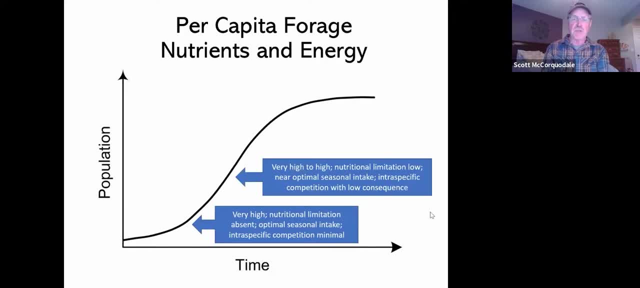 So what would be the leading factor here in this case is the number of animals that live within this. ungulates is pretty minimal As we move up the curve. it's still very high to high. Nutritional limitation is still pretty low. It's not absent. perhaps We're still getting pretty good seasonal. 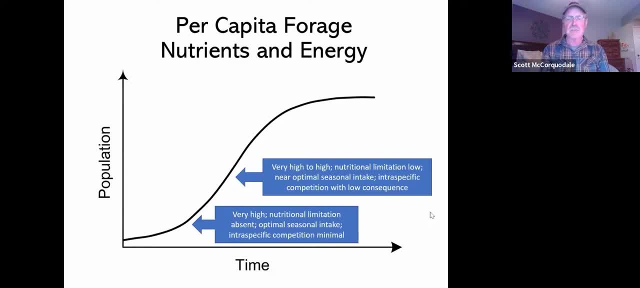 intake of nutrients and energy And interspecific competition may be occurring, but it has pretty low consequence. When you get up to here, things have changed a lot. The per capita forage and nutrients energy is low. There's a strong nutritional limitation occurring Seasonal. 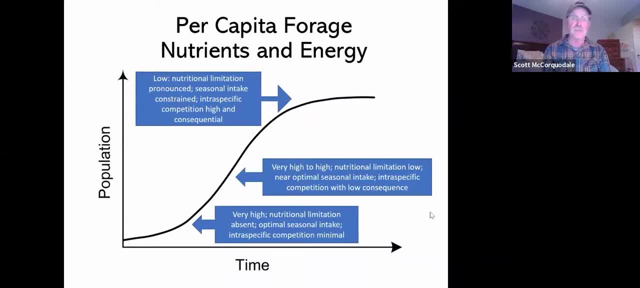 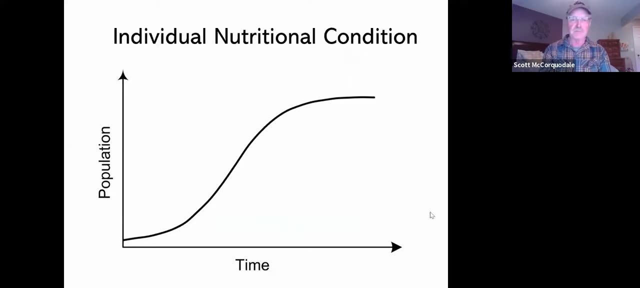 intake can be dramatically constrained And this individual-to-individual competition within the population can be really high and is of consequence. So there are distinct winners and losers in this game. Individual nutritional condition: Animals during colonization. they're in excellent shape. There's low variability. Everybody's doing well. 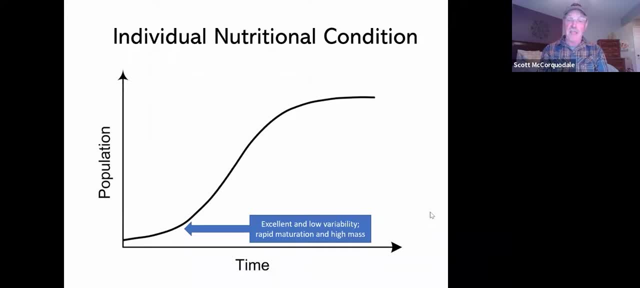 Animals typically grow very fast and they reach pretty large adult mass. for that particular species In this part of the curve it's still excellent to very good. It might be a little bit lower for animals that are lactating during the current year but they're still doing pretty good And of course, by the time you get up here, 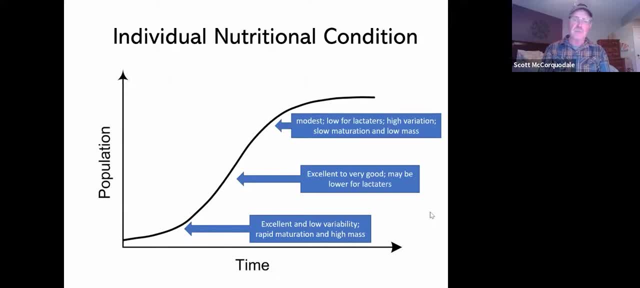 when you start incurring density dependence, that becomes modest. It becomes pretty low for lactators because of the energy demands of lactation. There can be high variation among individuals. Animals typically grow slower and a lot of times they won't be sort of on the high end of mass for that particular species. 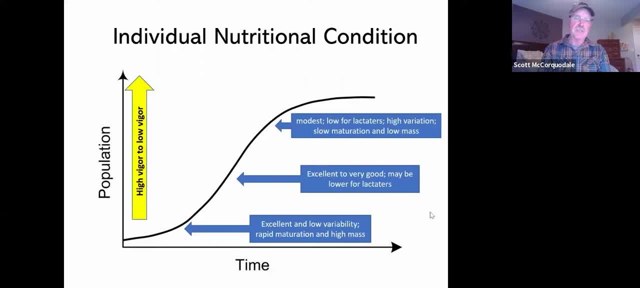 If you, as you're going up this population size, with the curve, basically transitioning from really high-vigor animals at the low end to pretty low-vigor animals at the high end or at the high density, Similarly, well, it's pretty common to see reduced antler and horn growth. as we move up there, Antlers and horns are 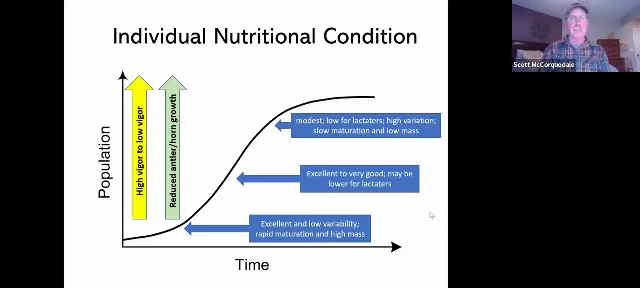 secondary sex characteristics. so they're not critical for survival but they are critical for sort of competition in the breeding competition. But when animals are sort of faced with this trade-off, they'll start investing less in antler and horn growth And of course the fat stores. 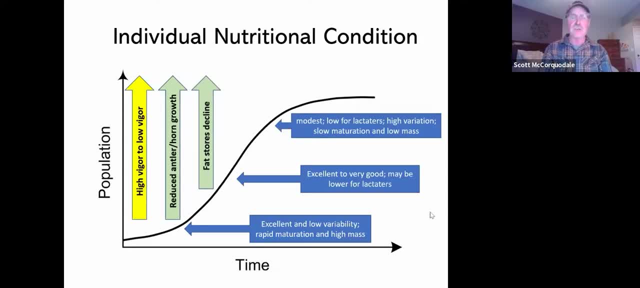 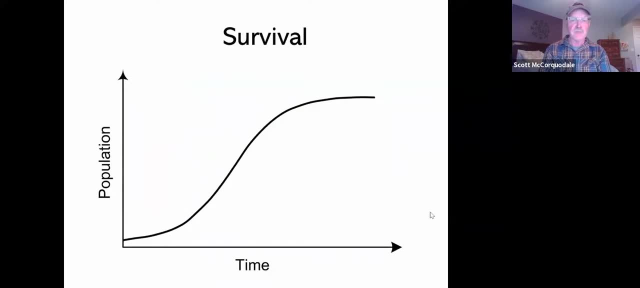 that the animals are accumulating during the good part of the year they're going to start declining From low density population to high density population. Survival, individual animal survival, colonization. it's excellent for adults. It can be really still pretty good for neonates and juveniles As the density increases. for time it'll still be very 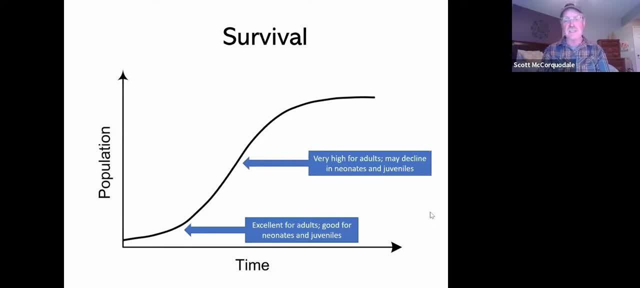 high for adults. It may start to decline in neonates and juveniles, but really not until you start getting into that inflection And then up here survival is can be still high, but it may also be modest for adults, depending on. 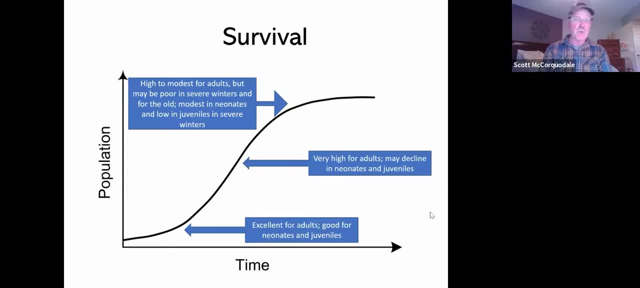 how strong the density of dependence is, But it may be poor in severe winters and for the older animals because they tend to be in a little poorer shape. It's typically modest in neonates and pretty low in juveniles during severe winters. Productivity: 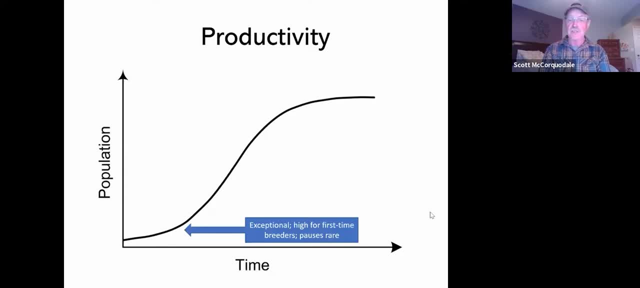 Exceptional In colonization High for first time breeders. So for example in elk the first time breeder is typically a yearling. In colonization phase yearling pregnancy rates can be really quite high. Pauses are rare, So when I say pause I'll use that term several times. So pauses. 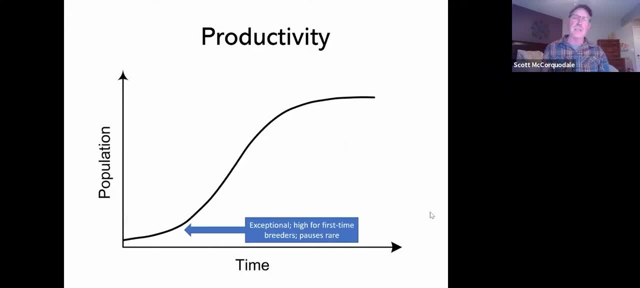 are a phenomenon. So these most ungulates in North America, if they're on a relatively high nutritional plane, they can pull off reproduction every year. even if they raise their young throughout the whole season all the way to weaning, it's still there. there can they are. 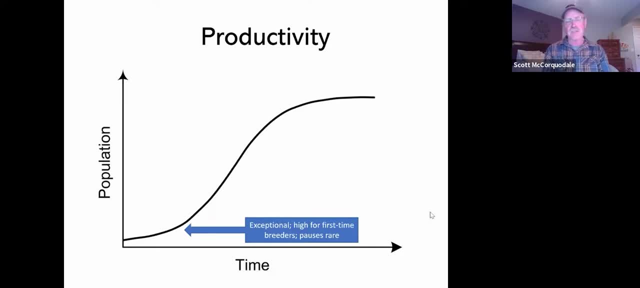 able to recover condition during the rest of the summer and the early fall and they're able to breed again, and so in this phase they they incur those costs pretty easily and recover pretty well. and so pauses, meaning skipping a year of reproduction, is rare. productivity is still high during the sort of eruption phase. it can be still pretty good for. 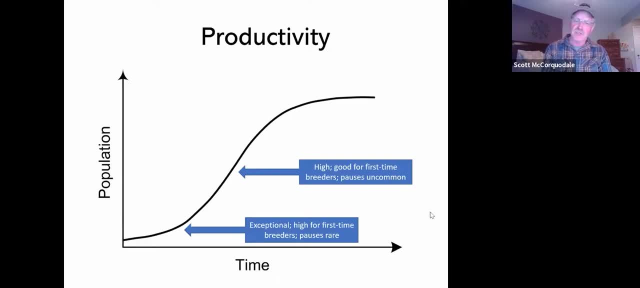 first-time breeders and pauses are still going to be relatively uncommon, but when you get up here where density dependence is sort of it's exerting a strong influence. pregnancy overall can be reduced and reducing recruitment. here's where you start to see animals that are typically a little 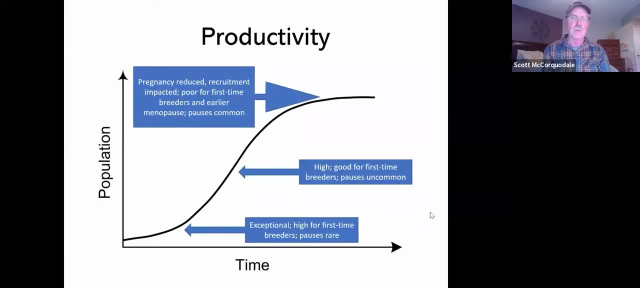 less productive, like yearlings again, or really old animals, for it can be. it's going to be lower, so yearling elk in a population that's operating in a strong density dependence, it's not going to be nearly as high as it was, you know, at a. 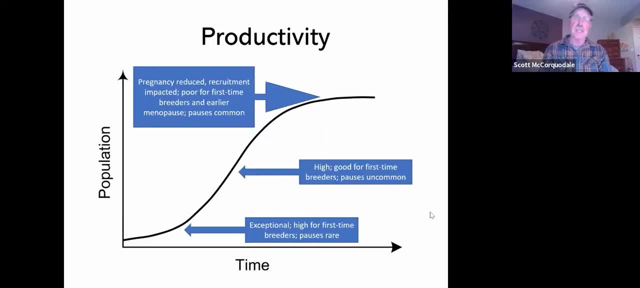 lower density and up here pauses can be common. so animals that successfully raise a young animal through the whole season and wean it, they're just unable to recover the full condition that they need you, you to be able to be, uh, productive again on the next cycle, and so a lot of times they'll end up. 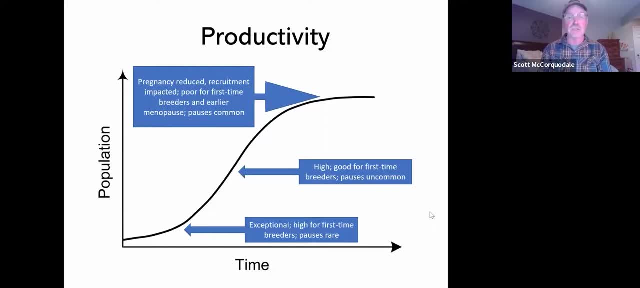 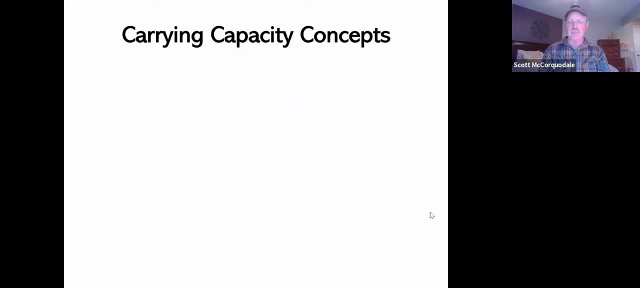 you know, skipping a breeding season and they'll have sort of alternate year reproduction. so that k that was on that curve is typically, it's been defined as the ecological carrying capacities is another way of thinking of it- ecc, and it's it's this sort of limit imposed by resource availability. 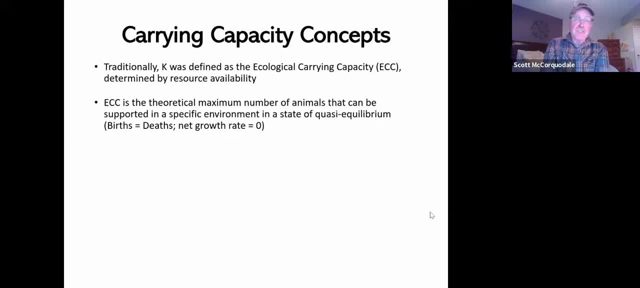 as a definition. it's the theoretical maximum number of animals that can be supported in a specific environment in a state of quasi equilibrium, and when you're at an ecc bursts by definition equal death and the net growth rate is zero. that's that flat part of the 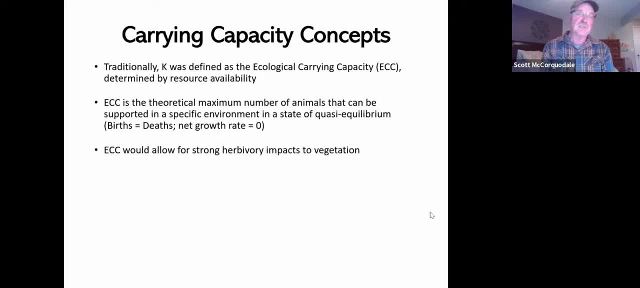 curve ecological carrying capacity does not prevent strong herbivory impacts to vegetation. so at high density the animals can actually degrade the habitat什麼 the habitat? They can impact the vegetative growth patterns of the forage plants and you can actually have essentially damage to the sort of forage environment. It's not a 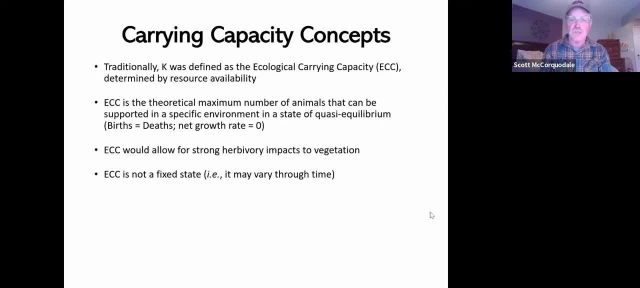 fixed state. It varies seasonally, almost always, and it can vary through time based on weather and sort of climatic effects. There's this interesting relationship between the animals and ECC. ECC shapes the animals and the animals shape the ECC via feedbacks and that adds to the 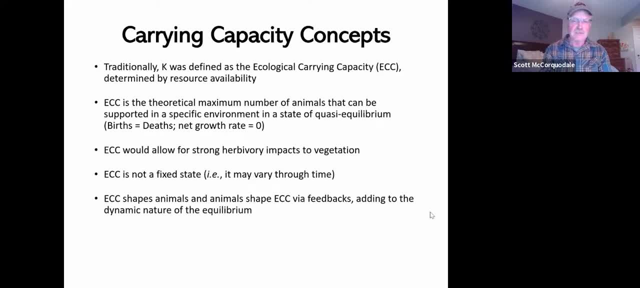 dynamic nature of the equilibrium. In range management there's a sort of a different concept, and carrying capacity is generally defined as the number of animals or use that can be supported without degrading the plant community. They're not exceeding a specific level of utilization. So if you're a range manager, 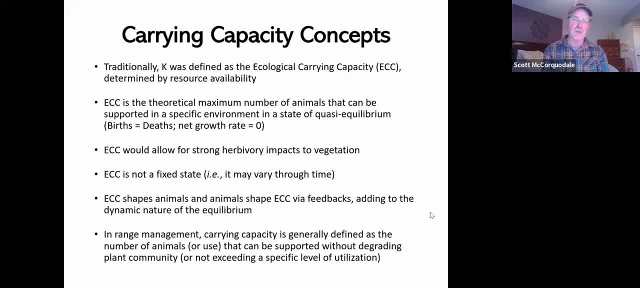 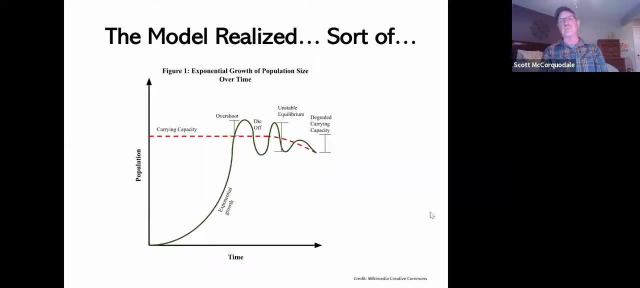 you're really trying to sort of make sure that the number of animals that are on the landscape are not more than the habitat can support, without loss of condition of the plant community. So that's a simple model, The way it sort of may play out in the real world. 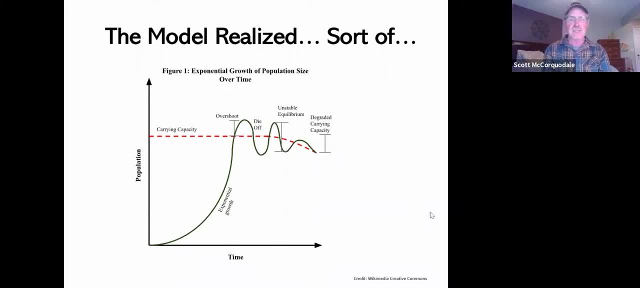 is a little bit different. So instead of it being this nice smooth, exponential growth, you've got this sort of inflection point and then you get this nice flat, straight sort of equilibrium at carrying capacity. it often looks more like this: So the animals may overshoot carrying capacity. That will. 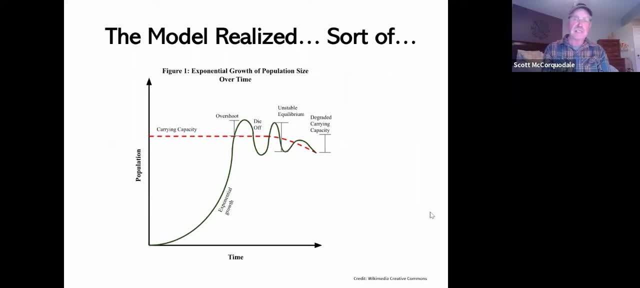 have an impact. The animals will die off, typically in winter. There may be degradation of the plant community. So you can see that carrying capacity dotted red line, It sort of changes, It goes down with time And so you kind of get more of this, you know. 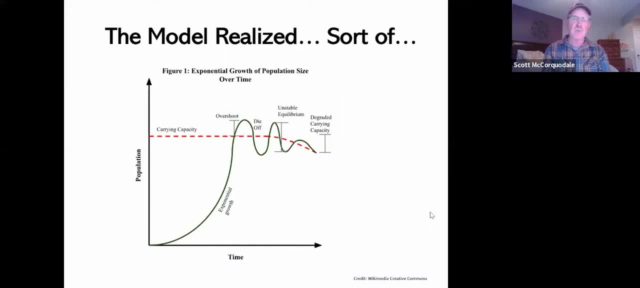 with sort of the classical oscillation, where the animals sort of overshoot and then they density is reduced, And so then the plant community responds, the per capita energy and nutrient intake increases again, the animals grow, and then they just kind of do this over. 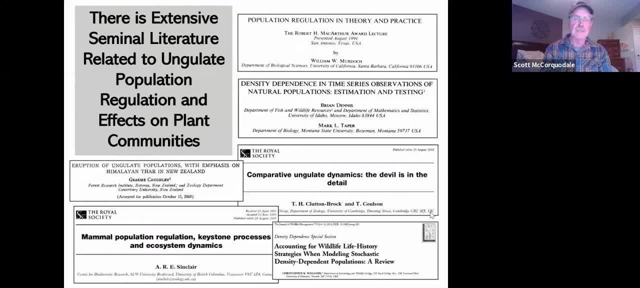 and over again. Okay, Okay, Okay, Okay, Okay. So this whole subject matter about population regulation and plant community effects from grazing guilds. it's a really extensive and very interesting body of literature And there's some really really good papers written by some really really smart people that explore. 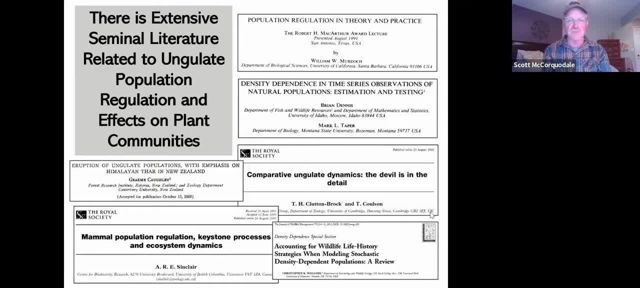 these topics in detail And I've just put on here just sort of a smattering of some of the things that are out there. Okay, And we can certainly anybody that's interested in this sort of this kind of stuff- we can help guide you maybe to some some pretty informative pieces. 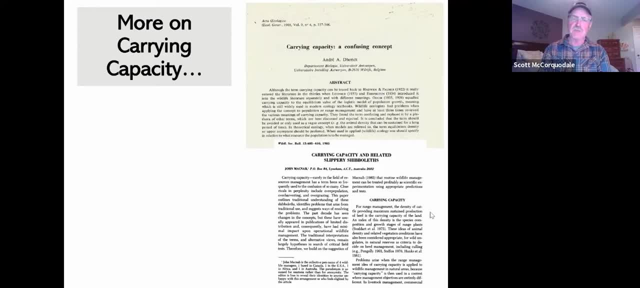 A little bit more on carrying capacity. As you can see from the sort of the abstracts of these two papers I posted to the right it's, it's got kind of a mixed review in the literature. It's a. I kind of think of it as carrying capacity is a little bit like. 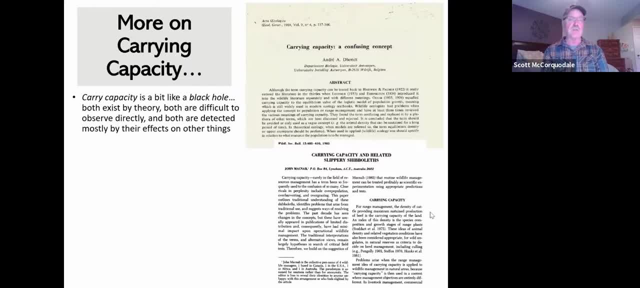 a black hole. But this sort of thing is kind of a black hole. I mean, Both exist by theory, both are difficult to observe directly and both are detected mostly by their effects on other things. And by black hole I mean this sort of, you know, astrophysics. 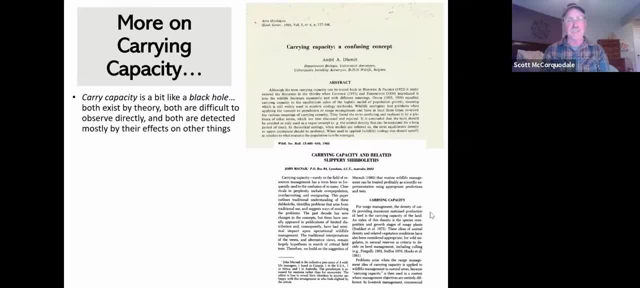 thing where a stark collapses on itself and eventually creates this sort of vacuum that sucks anything in its vicinity. You can't see it with a telescope, but there are other ways that astronomers detect them. It's really difficult to estimate ecological carrying capacity finitely. You know, early attempts were just like: if you know how much biomass is produced in a landscape, you can you know sort of how much each animal would need. You can kind of do some math. That ought to work out right. 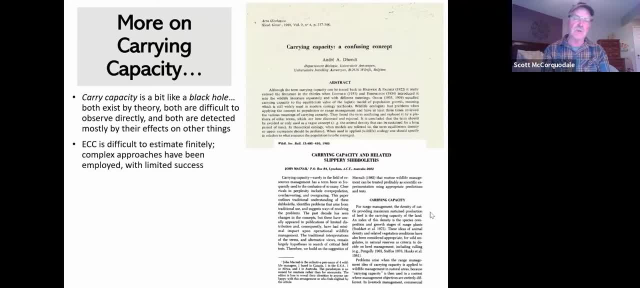 But it doesn't work out very well because it's more complicated than that. More complex approaches have certainly been developed and there's a lot of published papers documenting those attempts. Those have fared better, but it's still a really difficult thing to finitely estimate. 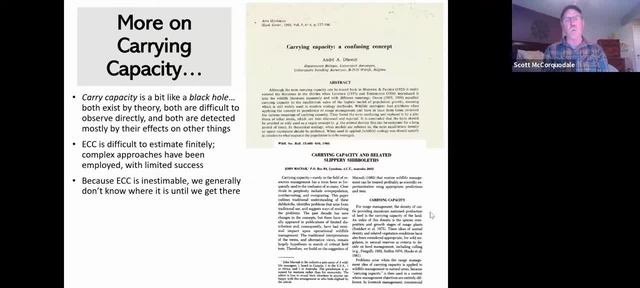 Because of that, we generally don't know where ECC is until we get there and start to see these sort of strong effects that are observable. Again, it's dynamic, It varies seasonally, It varies across years And this is an important point. 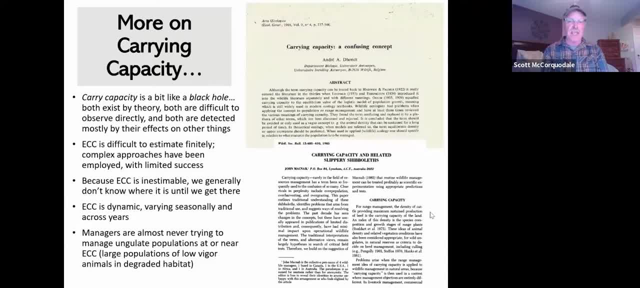 Managers are almost never trying to manage unneeded populations at or near ECC. Those would be large populations, low vigor, animals in degraded habitat, And so that's really almost never the goal. I mean, I guess you could argue that sort of the Park Service's natural regulation paradigm is kind of that. 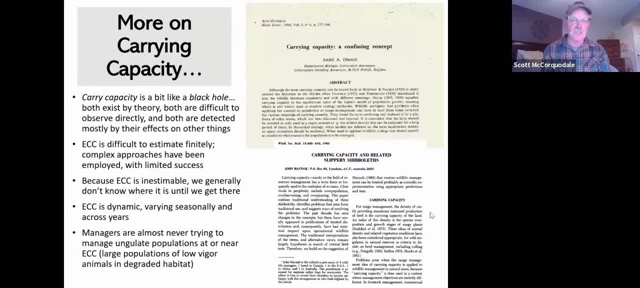 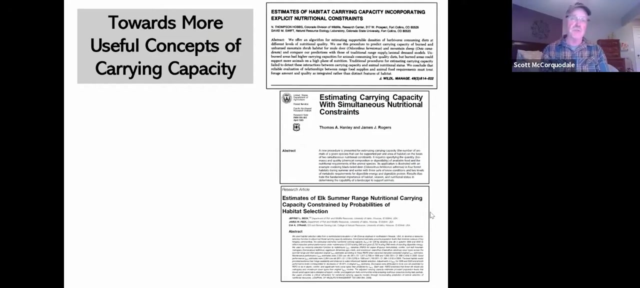 But you know, most agencies that are that are managing, for example, for hunting, they're not going to be at all trying to manage populations to this point where they're really under strong density-dependent effects. So there has been work done towards developing something that would be potentially more useful. 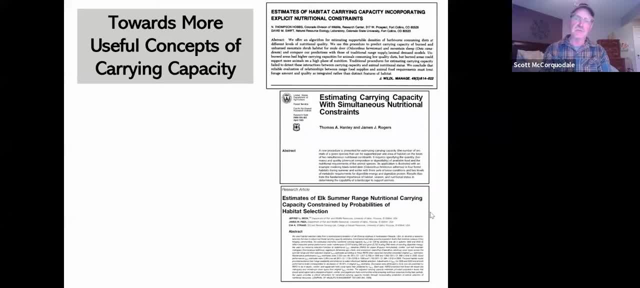 as a concept of carrying capacity than sort of the straight-up K or ECC. So ecologists and resource managers have promoted- and we've done a lot of work on that, It's kind of a redefined- concept of nutritional carrying capacity. This concept focuses on the number of animals a landscape can sustain in a desired nutritional state. 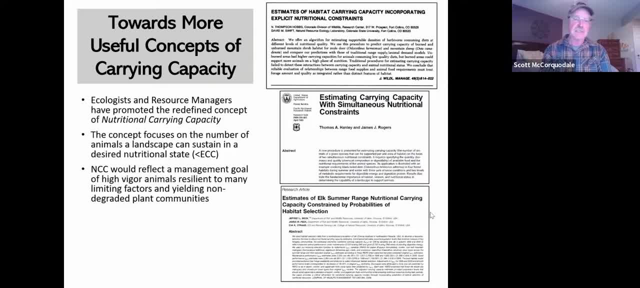 And that's going to be something less than ECC. Nutritional carrying capacity would reflect the management goal of high vigor animals resilient to many limiting factors and yielding non-degraded plant communities And, of course, not just forage biomass but also animal forage. 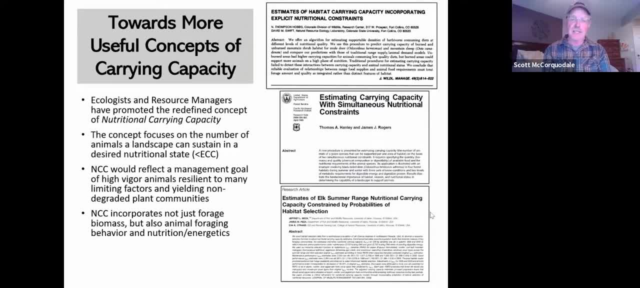 Foraging behavior and nutrition energetics. Animals will not eat a diet of only one kind of forage- Wildlinglets just will not do that, And they will also be reluctant to forage in certain biomass settings, even though there's the right species there. 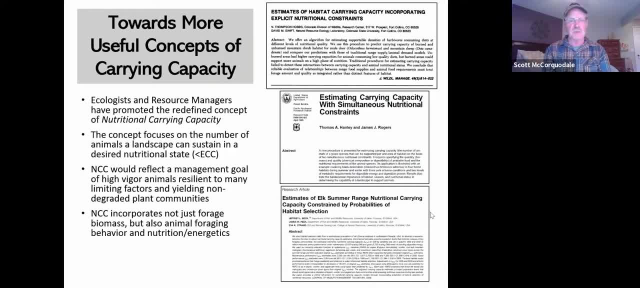 It's just inefficient and so they're pretty reluctant to do that. So you have to sort of incorporate this behavioral aspect about how animals select forage and use forage To better kind of approach the nutritional carrying capacity problem It's difficult to estimate and approaches that have been used. 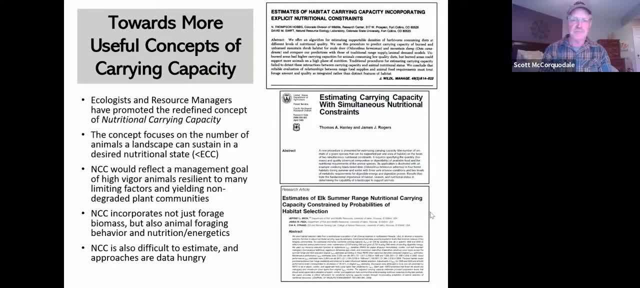 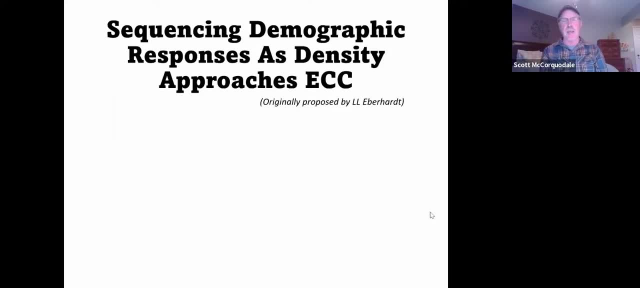 and promoted, are pretty data hungry, So let's shift gears a little bit. So let's talk about what happens with demographic parameters as density approaches ECC, And what's going to be on the rest of this slide are is an idea that was originally proposed by the late Lee Eberhard. 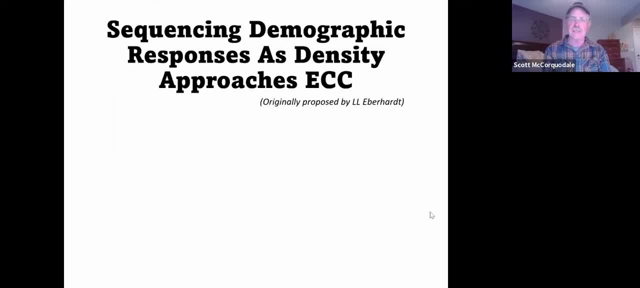 who was a really kind of world-class ecologist, And so the first thing you'd expect to see, as you get stronger and stronger density dependence effects, is that juvenile survival is going to decline. Usually that happens during the winter. You're going to see increased age of first reproduction. 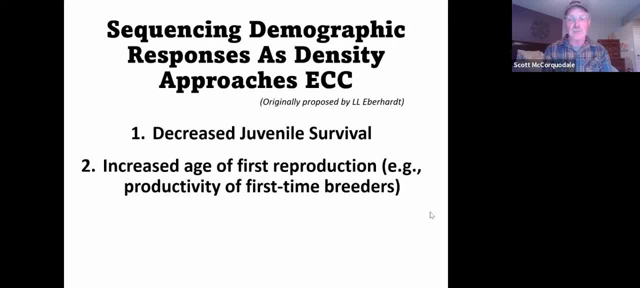 So, again as an example, using yearling elk as first-time breeders, the pregnancy rate for yearlings is gonna decline as density dependence starts to operate more prominently. Eventually you get decreased age-specific fecundity, and fecundity is a word that's on that glossary. 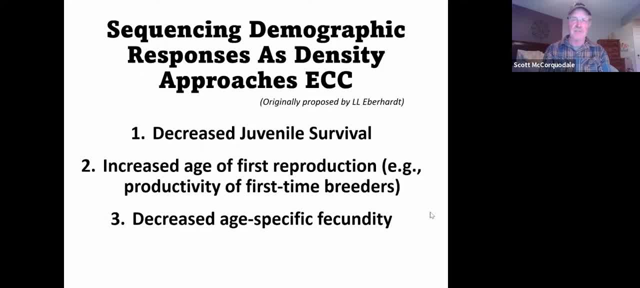 But it's essentially, it's a term that reflects the productivity of the individuals in the population. And then, lastly, the last thing you'll see is decreased adult survival. If you remember, from that survival slide, it said that survival in adults continues to be pretty high. 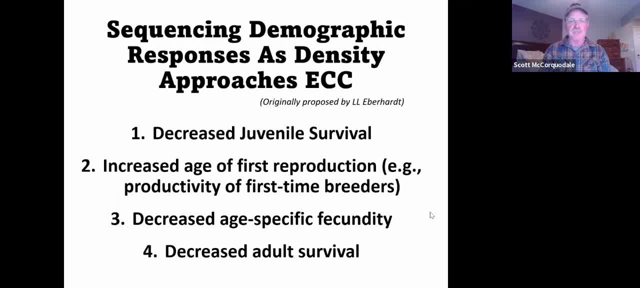 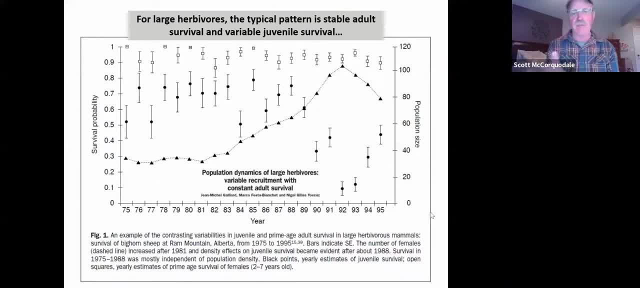 through the whole cycle of that logistic model. This is a really informative graph. I mean it looks maybe intimidating a little bit at first, but there's a lot. all these pieces of the story are on this one graph. So the thing that kinda looks like a side view of a mountain. 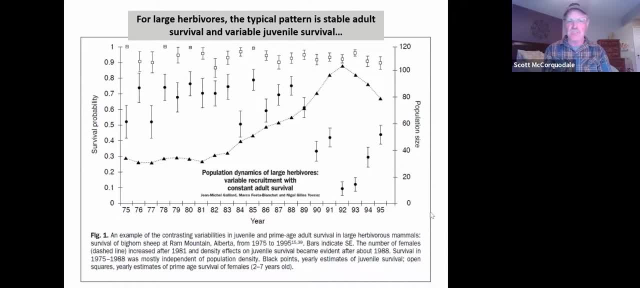 with the little triangles. so this is a population of bighorn sheep in a place called Ram Mountain, which is in Alberta, And so that's what the population was doing. It was increasing and then, as you move to the right, 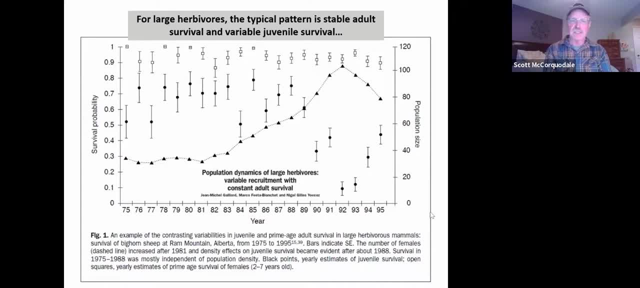 it got to a point where it started to decline- The little open squares at the top that you see going along there. that's adult survival and, as you can see, adult survival stayed pretty constant through this whole cycle And what that graph of what the population did sort of suggests that they did sort of surpass. 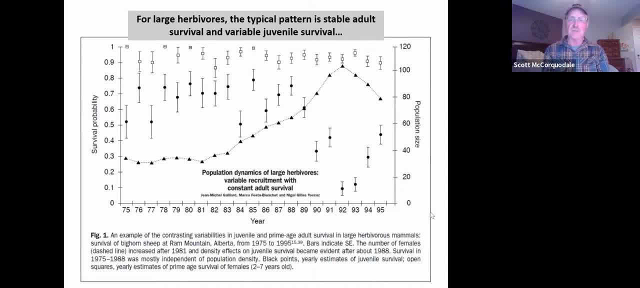 carrying capacity at about 92. But even though they did do that, the adult survival remained high. The little black dots. that's what happened with juvenile survival And you can see that that stayed relatively high as the population increased. But when it got to pretty high. 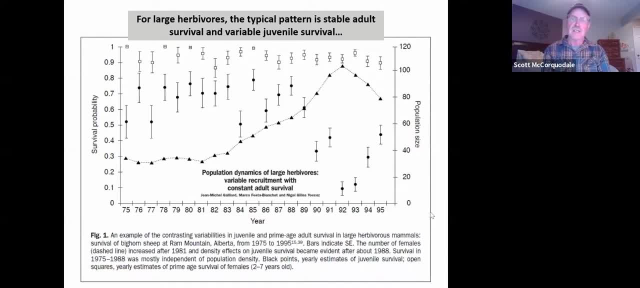 density and as particularly as it moved over the top of what was presumably carrying capacity, that began to decline And it's really apparent in that figure. So you can see this figure with what the population did, how adult survival stayed relatively constant but juvenile survival did. 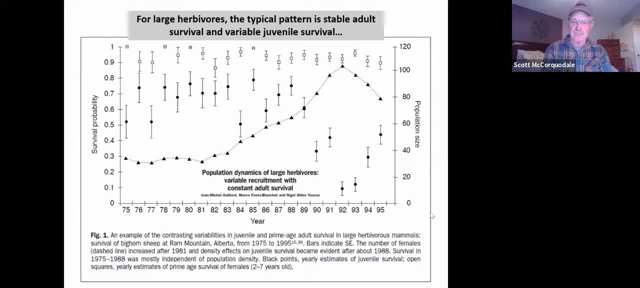 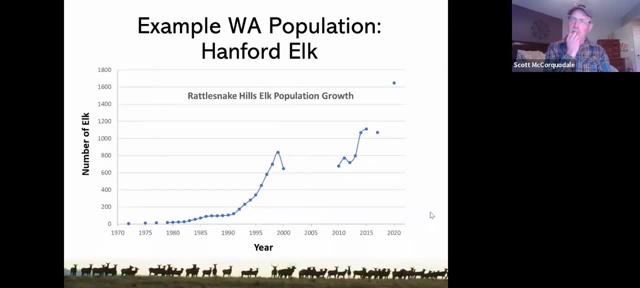 not. Juvenile survival started to decline pretty substantially. So most of the time, with most populations, we don't really know where we're at on this curve, right? I mean, we didn't see them start. We are at some place on that curve. We might know if we're. 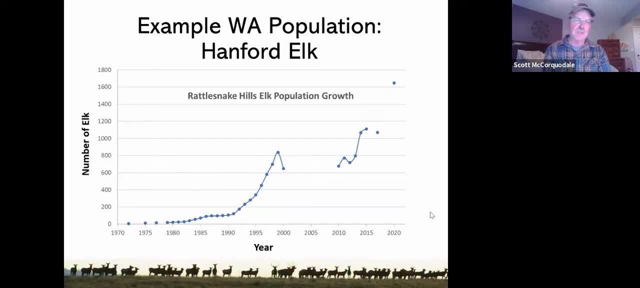 kind of up there where carrying capacity and strong during density of dependence is operating. But we really don't usually see populations from their origin. But there's a couple of good examples in Washington where we have, And one of them is elk occupying the Hanford nuclear facility near Tri-Cities, also known as the Rattlesnake. 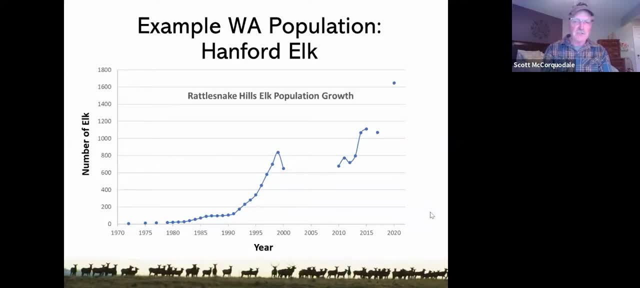 Hills elk population And this population was created by about five individuals, we think that walked into the site in about 1972 during the winter. Everybody expected them to go home after the winter ended but they didn't. They stayed and started to grow slowly and essentially. 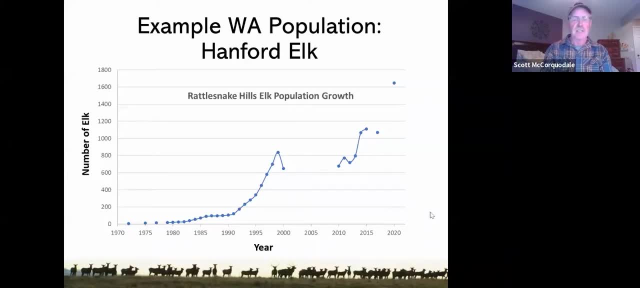 established a resident herd on Hanford, mostly on the Aradalands Ecology Reserve part of Hanford. So this little yellow arrow is me starting my master's thesis work. So I came to Washington originally as a graduate student to do research on this Hanford elk population. 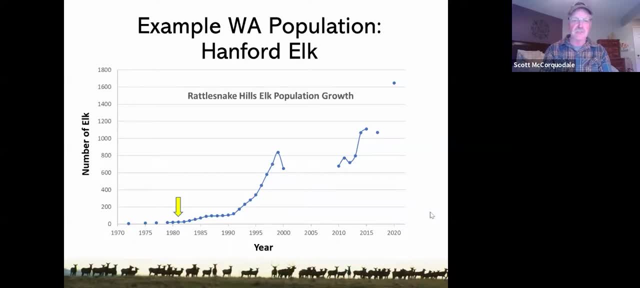 And when I started in 1982, there were 27 elk in that population. There had been no studies, but there had been no studies previous to that. So we were kind of looking at this thing at the beginning And also, you know, what made the project happen was that these elk were kind of living in a place that 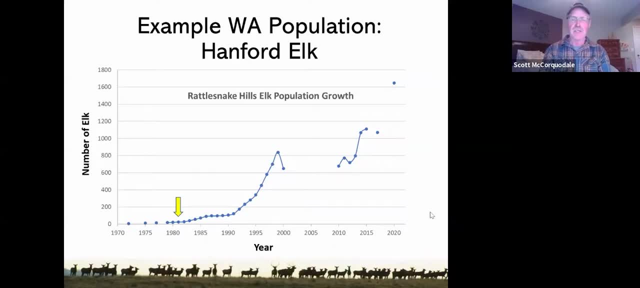 the current thinking about elk said should be pretty hard for them to do. But as you can see through this time cycle up through last year and on this graph, this population kind of did what we saw from the logistic curve. It grew slowly and then it reached this inflection point where 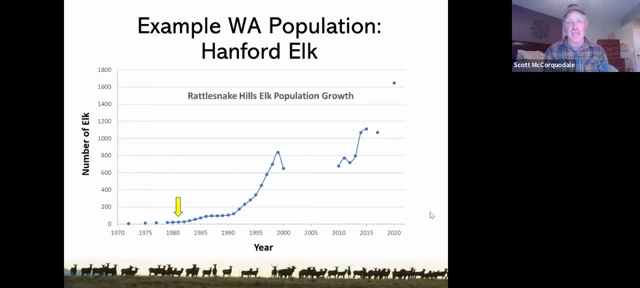 you had enough animals that the exponential effect started to be pretty dramatic. It grew rapidly. You know a lot's happened so there's some missing data there. There have been surveys every year after about 2000.. For a while there weren't surveys. Animals have been removed. 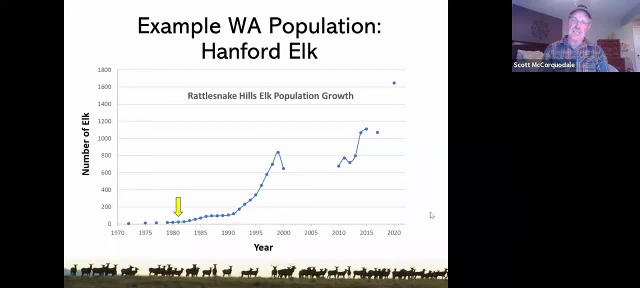 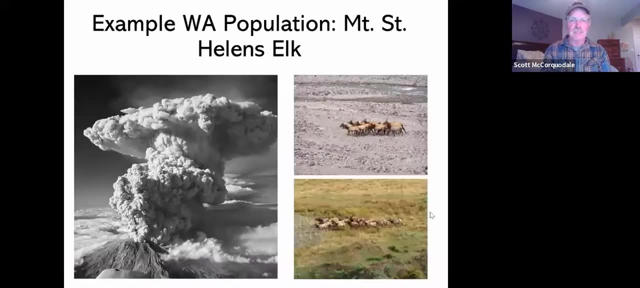 various ways from this population. so it doesn't look exactly like the logistic curve, but you can see that that beginning part really follows that pattern pretty well. The other really good example happened at Mount St Helens. So in 1980, the mountain blew in May. 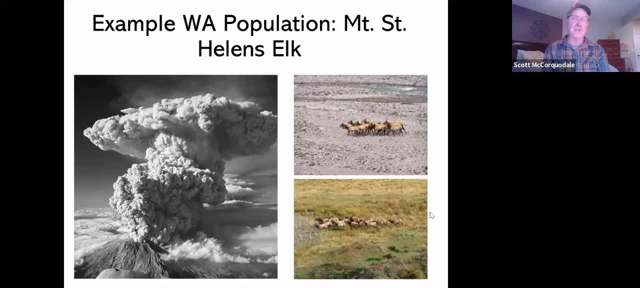 and in a certain part of that landscape every elk that was standing there died and was wiped away, Many of them almost vaporized, And so this area became part of it, became devoid of elk. but plant community succession occurred fairly rapidly in parts, and pretty soon, not very long after that, the environment started. 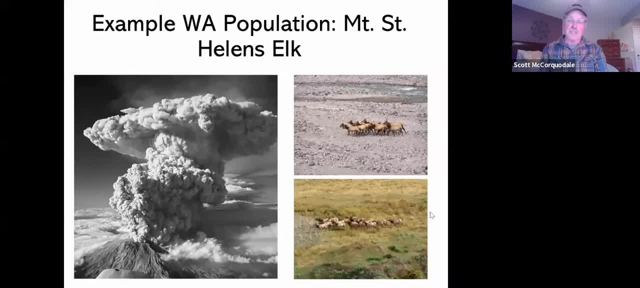 to be suitable again by elk, and elk started colonizing it by walking in from areas outside of the blast zone. A graduate student named Evelyn Merrill studied elk during this time. I actually helped Evie And so I was sort of out there again at this early stage. and then what happened at St Helens is 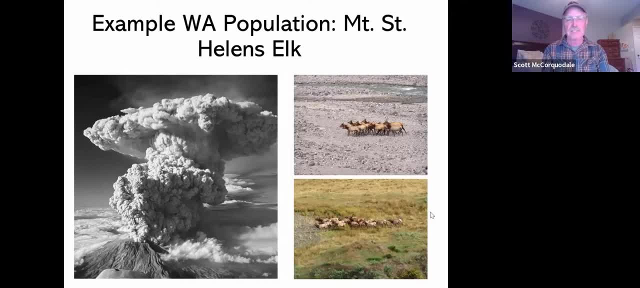 the elk population continued to grow pretty rapidly Because much of the landscape had been commercial forest. the owners wanted to get back into production and so there was a lot of effort put into reforestation and so there was a lot of change in the plant community Early on before. 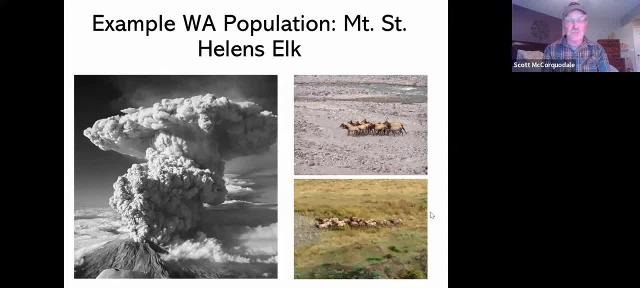 the sort of trees started to close in again. this was a really great place for elk to live. When I was out there with Evie there were fireweed plants that were eight or nine feet tall. All those nutrients that had been in the forest and all the critters in the forest went into the ground as 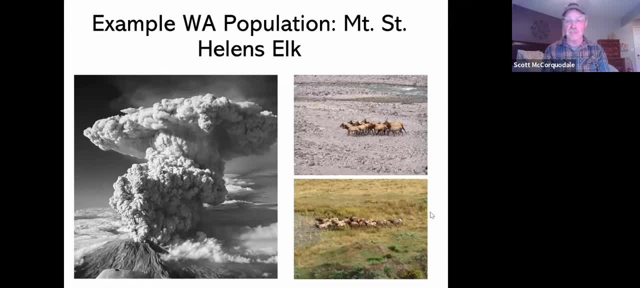 sort of served as fertilizer and it was a really productive, fast recovering environment and for a while it was like about as good of elk habitat As you could think of. But as the elk population grew and then the landscape started changing, 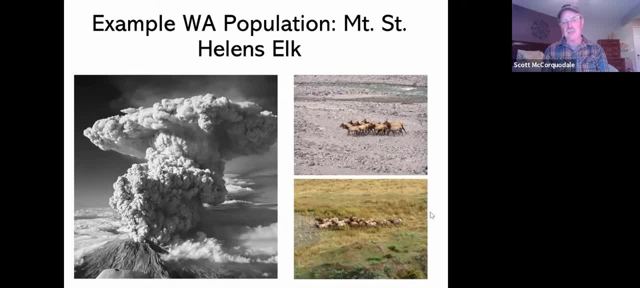 because the forest started closing in again, carrying capacity undoubtedly started going downward. while the elk population was going upward And by about the late mid to late 90s there were there were pretty becoming pretty obvious evidence that this population had probably overshot carrying capacity. 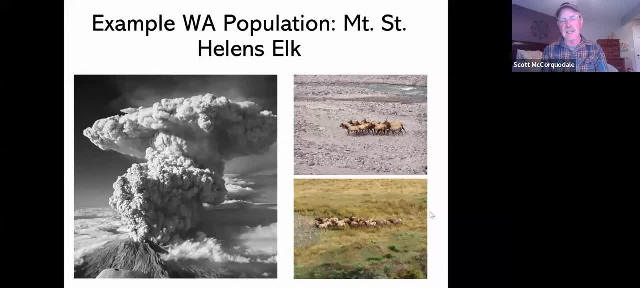 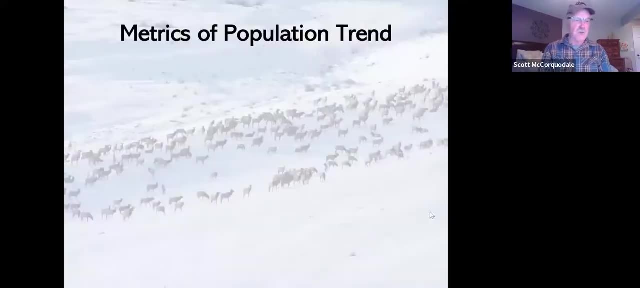 There was a lot of sort of winter mortality happening, And so we saw this phenomenon with this Mount St Helens recolonization event. That really looks very much like the logistic model. Okay, so again when we start reading literature and papers about what populations 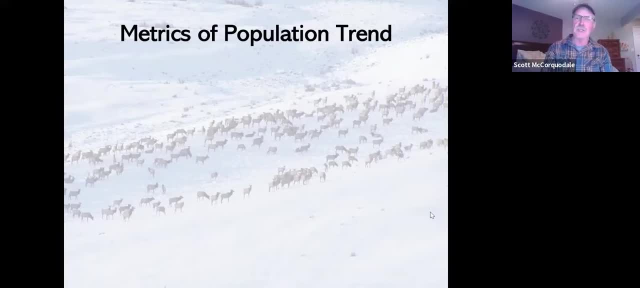 ungulates are doing. we're often interested in sort of: what is the trend in the population? How are the numbers changing in the environment, time And the way we do that is a couple of different metrics. One is known as the finite rate of increase, or what we call lambda, And that's a really simple metric. It's basically 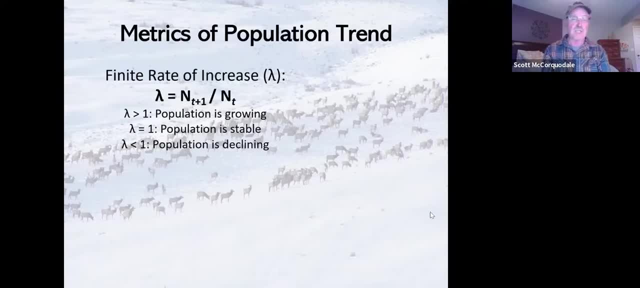 the number of animals at time, step t plus one, divided by the number of animals that were there last time. step Using lambda as an indicator of trend. if the population is the same, if it's nt plus one is the same number of animals approximately as the number of animals at. 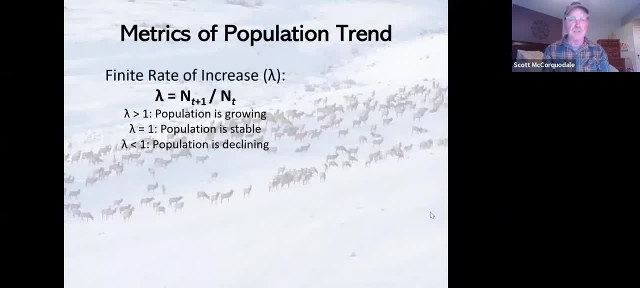 time t it's going to be one, right, So that's: lambda equal one is a population that is stable. Lambda over one is a population that's growing, and lambda less than one is a population that's declining. And you can derive from that another metric that's pretty useful, which is called the. 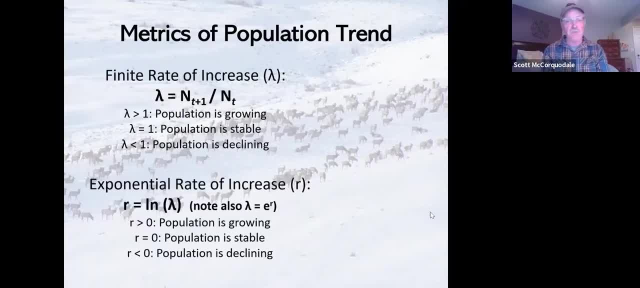 exponential rate of increase, which is simply the natural log of whatever that lambda value is. And it's this sort of re-centers the metric on zero. So a population with an r of zero is stable, not changing. If r is more than zero, the population is growing, And if it's less than 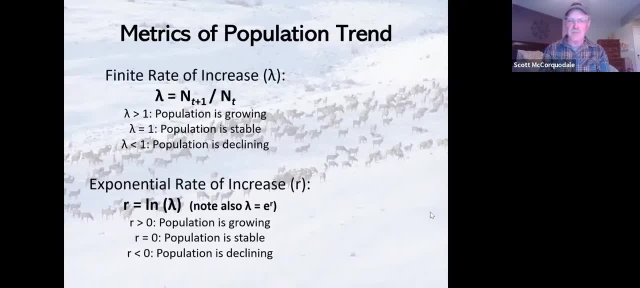 zero. the population is declining, And so, just to show you an example: so if we had a population that doubled from over a time, step the lambda, for that would be two right. So it's twice as many animals at t plus one as we had at t plus one, And so that's a population that doubled from over a. 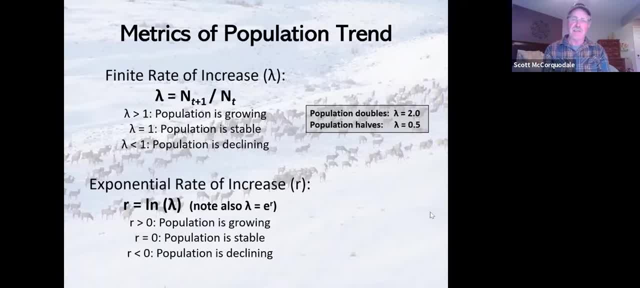 if it halved it would be 0.5, right, And so there's no, there's no counterpoint to this parameter that you just came back and happened. So, essentially, the- you know the magnitude of this is like two, or the inverse of two. 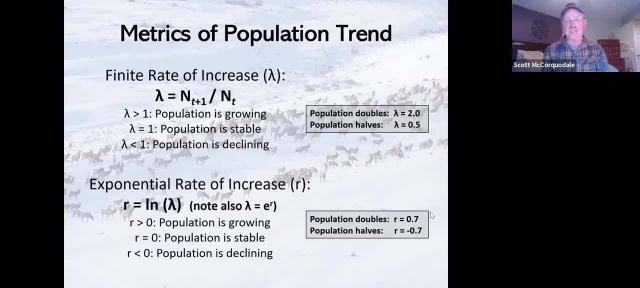 Interestingly, using r is the metric: if the population doubles, it's 0.7, if it halves it's minus 0.7.. And so for that reason, a lot of times, eventually, that population that causes is constantly finding r to be more useful. 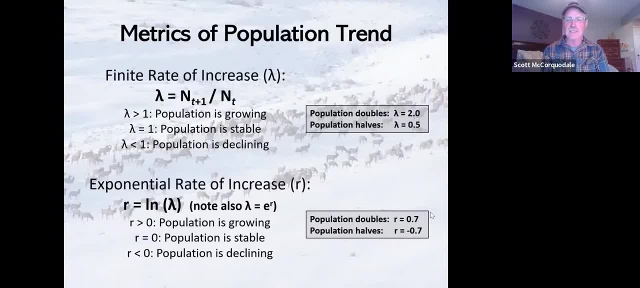 and more easily interpretable metric for trend, because if you have sort of similar magnitudes of change, they're going to be the same, just differing by sign, whereas the lambda. you kind of have to think about it a bit more because it's not, it's not quite as intuitive by just looking at the lambda value. so 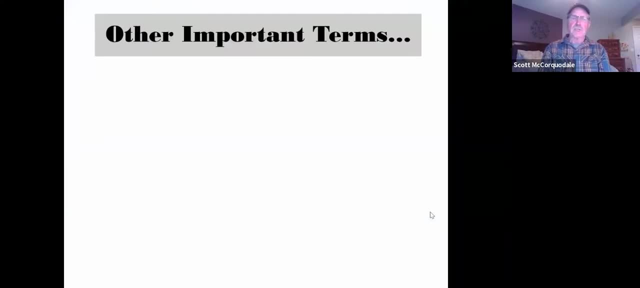 so just a few more important terms. these are on the glossary. i'm not going to hit very many of the terms that are on the glossary. we'd certainly be happy to answer anybody's questions at any point in time about anything that's on that glossary that we don't talk about today. we won't, we won't. 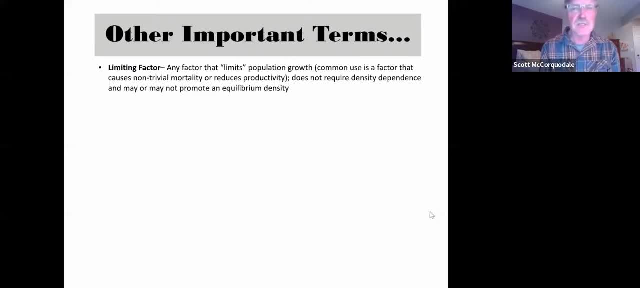 get to a lot of those terms today, but here's a few that i think are pretty important, and you will absolutely see these if you start reading the literature about ungulates and predation effects. limiting factor, limiting factors: any factor that limits population growth and its common. 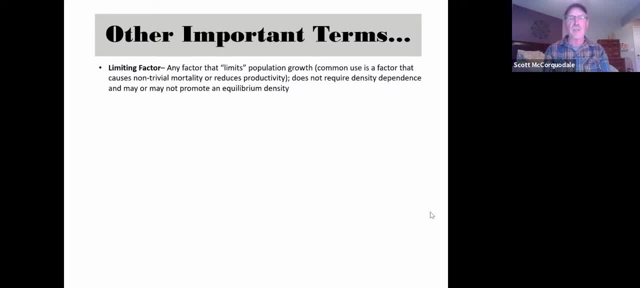 use is a factor that causes non-trivial mortality or in some way systematically reduces productivity. it does not require density dependence and it may or may not promote an equilibrium. density regulating factor is a limiting factor that affects population growth and has an effect that varies with density. a regulating factor typically facilitates population increases at